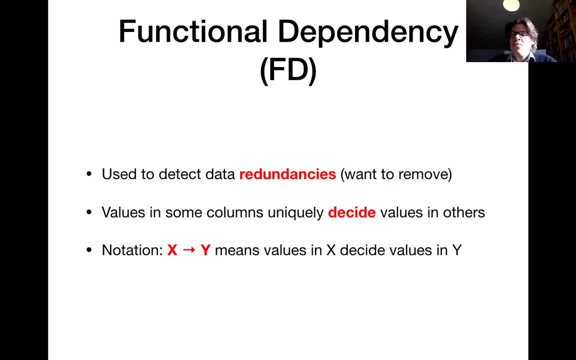 functional dependency just means that the values in some set of columns imply the values in some other set of columns. So you write them: x implies y, where x and y are sets of attributes, And the semantics is that if you know the values in x, then you also implicitly know the values in y And 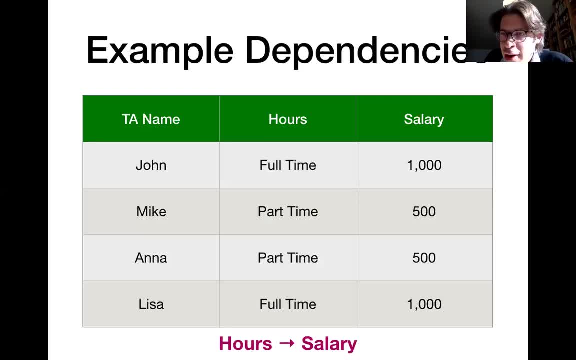 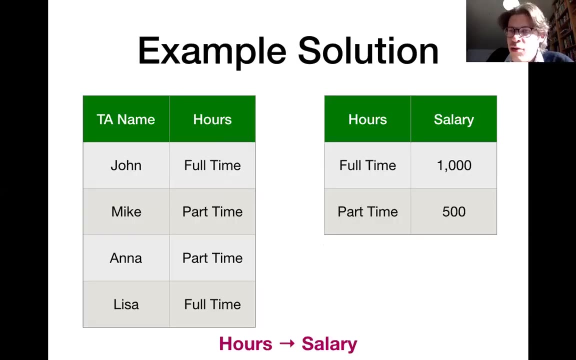 the semantics is that if you know the values in x, then you also implicitly know the values in y, And if you have those functional dependencies within one single table, it means that you could store redundant information like here, and that has various disadvantages. The solution is to decompose. 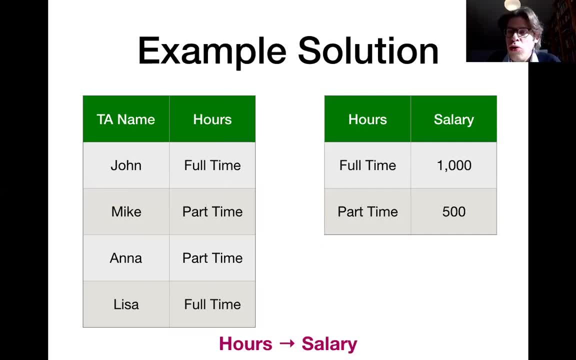 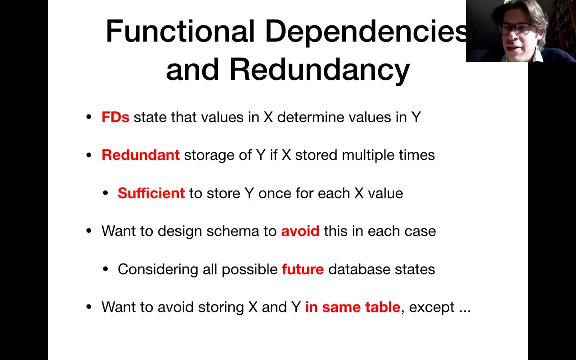 tables such that function dependencies do not hold within the same table anymore. And here we essentially resolved the redundancy problem. And here we essentially resolved the redundancy problem, All right. So we have discussed about function dependencies and we have discussed that they indicate. 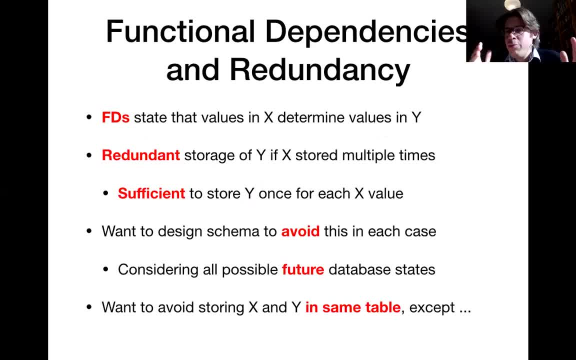 redundancy in most cases. One exception is if the function dependency essentially states that knowing the value in key columns implies the values in other columns. In this case you cannot have redundancy because in your database you can only store one row with the same values in the key columns. All right, 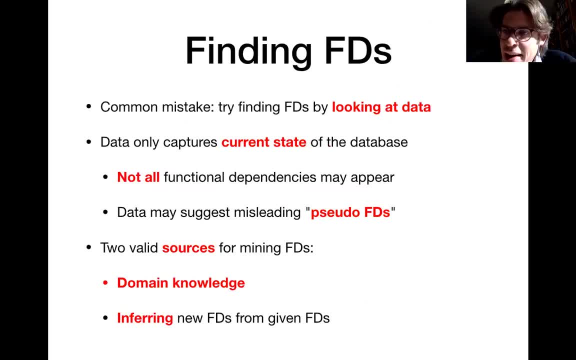 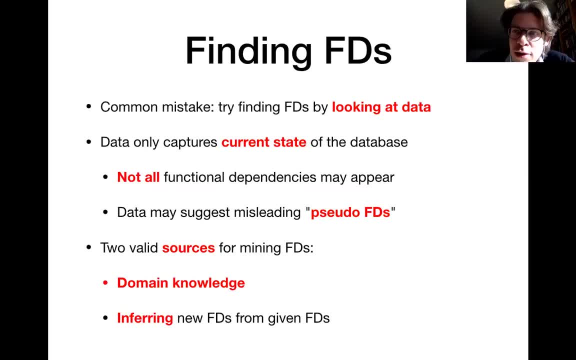 because that only represents the current state And even if it looks as if you have a function dependency there, it might not generalize. So valid sources for function dependencies is first of all domain normalization. If you just know from your use case analysis that this function dependency must hold, And based on some 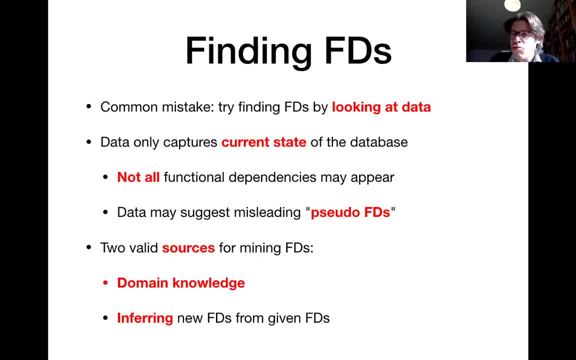 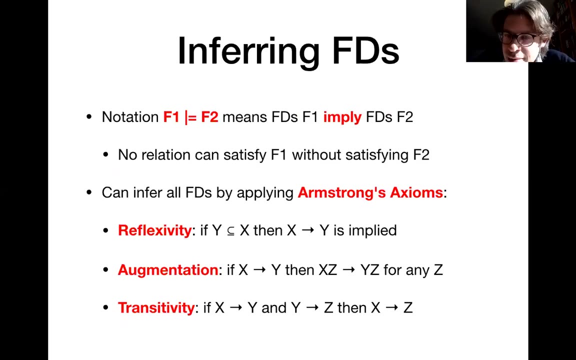 initial function dependencies derived based on domain knowledge. you can infer more function dependencies via algorithmic methods. Now, the last time. we have, in particular, discussed about Armstrong's axioms, which are a couple of rules that allow you to infer new function dependencies. 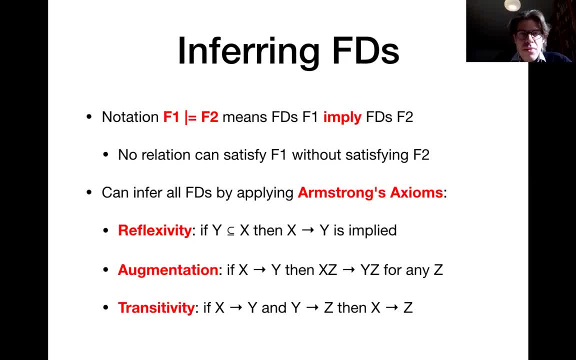 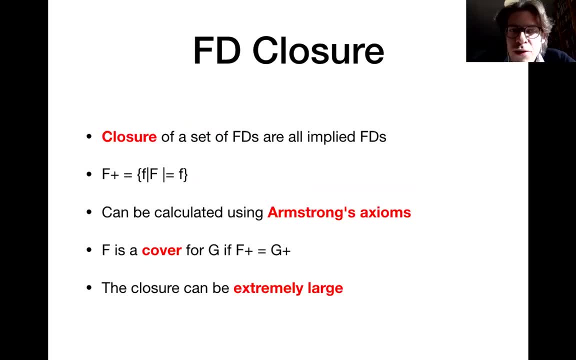 And if you apply Armstrong's axioms often enough, then in the end you end up with the closure for a given set of function dependencies, which is essentially all the function dependencies that can somehow be inferred from the original ones. Now, the problem with those closures is that they are extremely large, So it is typically impractical to try to. 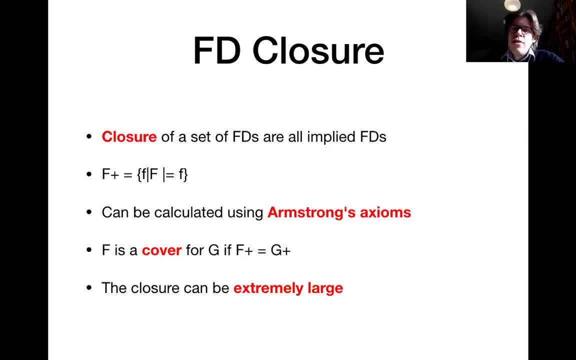 calculate one of those closures. So now in the following we're going to discuss how we can narrow down our scope a little bit and not try to infer all function dependencies, but rather only infer function dependencies that are based on the same attributes, on the left-hand side basically. 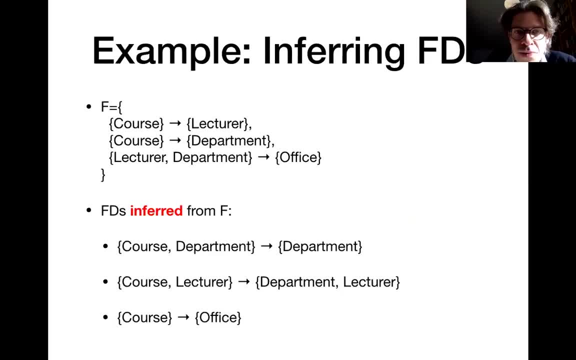 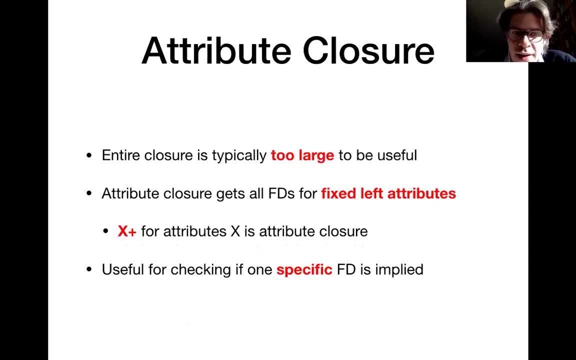 So this is one way of narrowing down the scope That leads to attribute closures. So an attribute closure essentially tells you what are the attributes for which I can infer the values. if there are no values for this set of attributes, So we typically denote that with the plus sign. 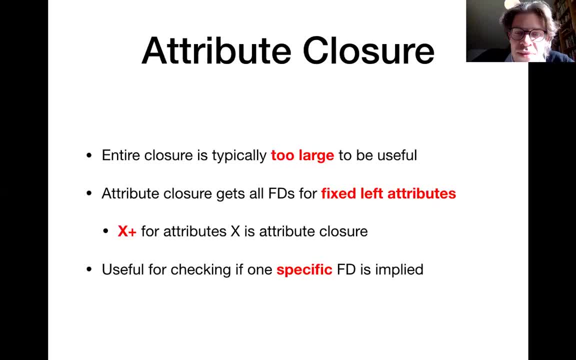 So if you have some set of attributes x, then x plus is the attribute closure for x, which means those are all the attributes for which you can infer values Based on the values in x using the function dependencies that you have. 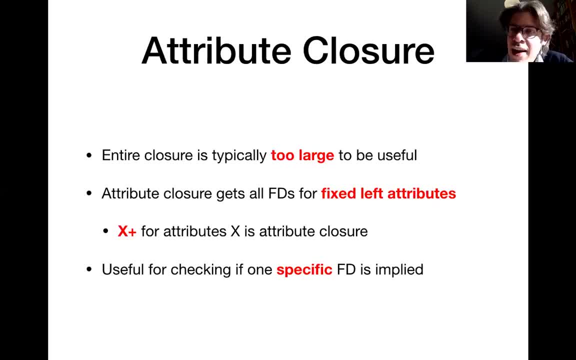 Now this essentially gives us some subset of function dependencies from the closure. For instance, you often want to check whether function dependencies which have specific attributes on the left-hand side, whether they can be inferred from given function dependencies, And the way to check on that is by using the function dependencies. 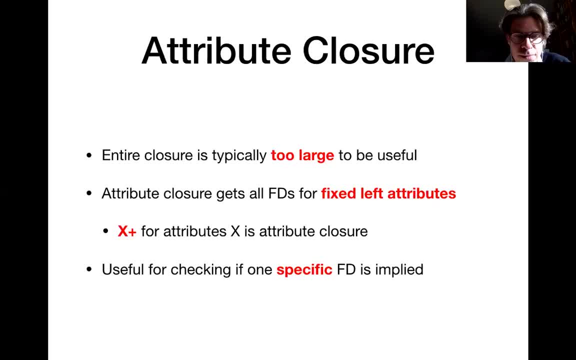 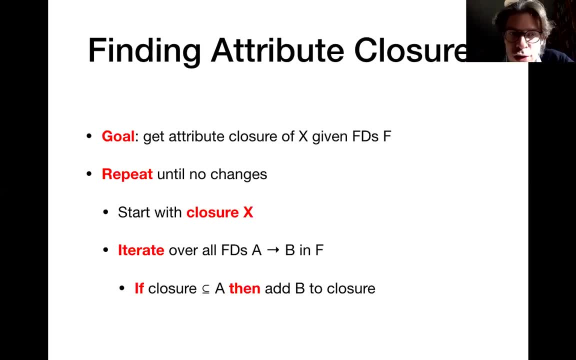 And the way to check on that is by using the attribute closure. Now, how can we calculate the attribute closure for a given set of functional dependencies? The algorithm is, fortunately, relatively natural. You see it here, And we essentially start with the attributes in x, because if I have given values for the attributes in x, 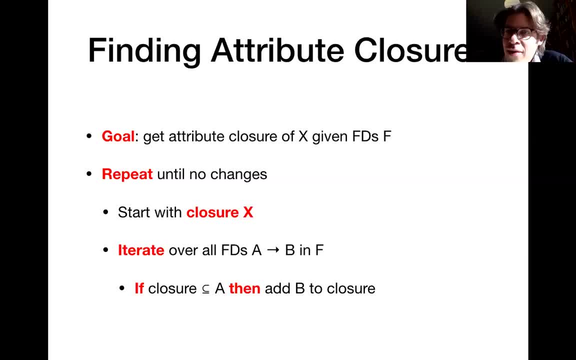 then most certainly I can infer the values for the attributes in x from that. Then I keep iterating and I keep adding more attributes whose value I can infer based on the given attribute values. So the way we do this is that we iterate over all functional dependencies which are of the form A implies B. 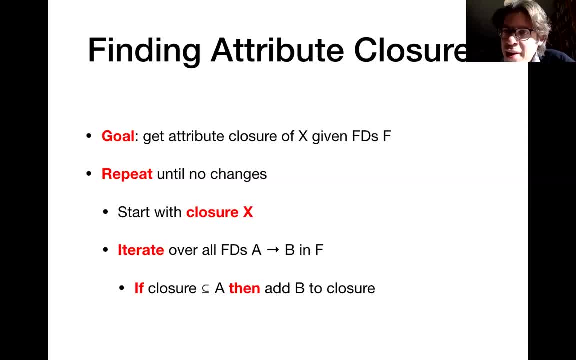 And if my current closure, meaning the set of attributes for which I can infer the value, is a subset of the, If it includes the left-hand side of the function dependency, then I add the right-hand side of the function dependency into my closure. 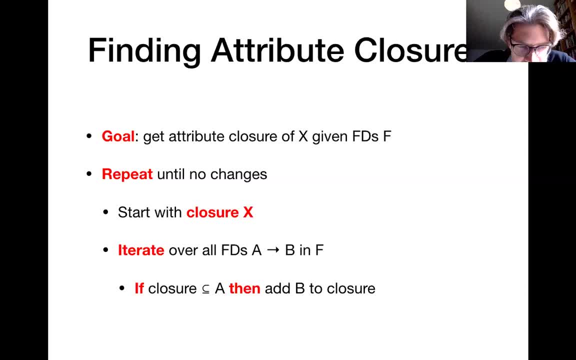 So this subset sign should actually be the other way around. So this subset sign should actually be the other way around. So if the left-hand side of the function dependency is included within the current closure, then we add the right-hand side to the set of attributes whose values we can infer. 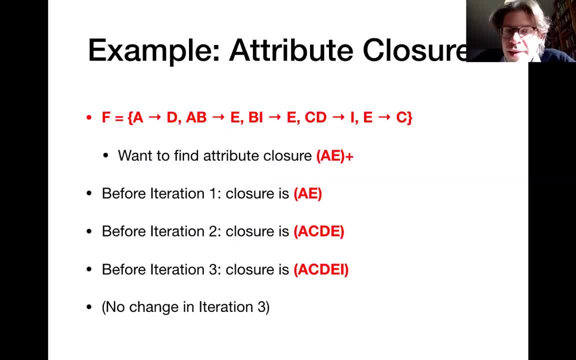 Let's make a little example in order to make things more concrete. We have given the functional dependencies in F, here on the top of the slide, And here we want to calculate the attribute closure of the attribute closure. And here we want to calculate the attribute closure of the attribute set A and E. 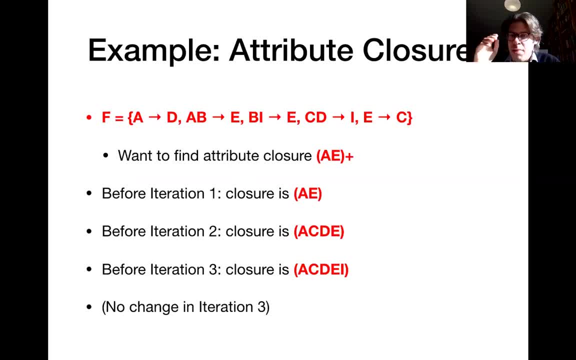 All right, so this is represented as A, E plus, And in the first iteration we just start with exactly this set of attributes A and E. So after we iterate over the function dependencies, we will expand that set by adding attributes C and D. 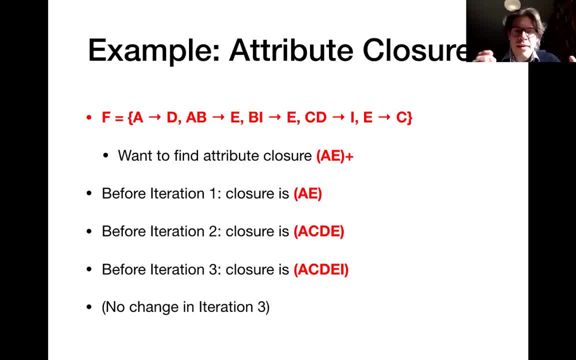 So let's see how that happens precisely. So during this iteration we assume that we have given values for attributes A and E. So if we look through the function dependencies, already looking at the first function dependency here we state essentially: if you know the value for attribute A. 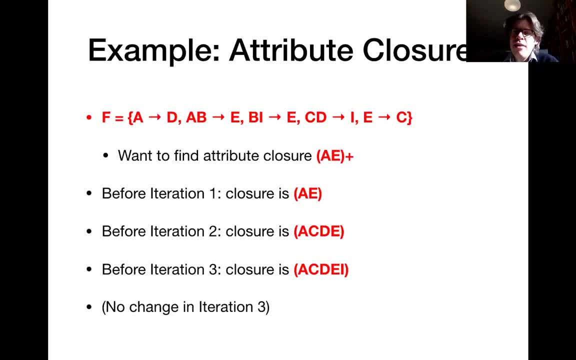 you can infer the value for attribute D. And since we know the value for attributes A and E, we know the value for A and we can therefore infer the value for attributes D And we can therefore infer the value for D. Now, going further through the functional dependencies here, 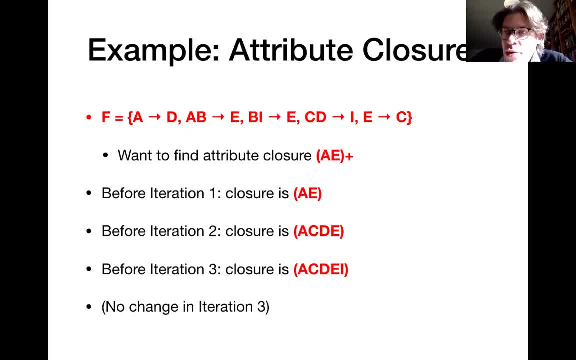 we see the last one, which essentially states that if you know the value for attribute E, you can infer the value for attribute C. And this is why, since we have given E, we also want to add C to our set of attributes that we can infer. 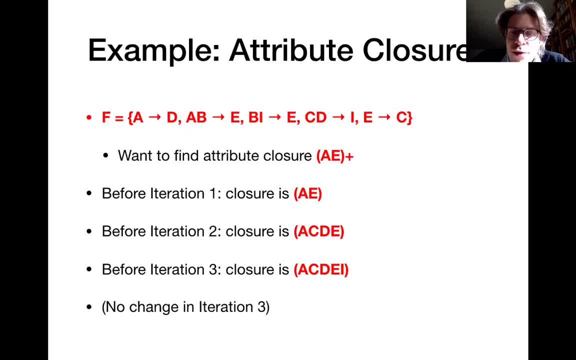 So after this iteration, we know that we can infer the attributes A, C, D and E given values for attributes A and E. Now we're going to iterate over the functional dependencies again, because we have just added attributes into our closure. 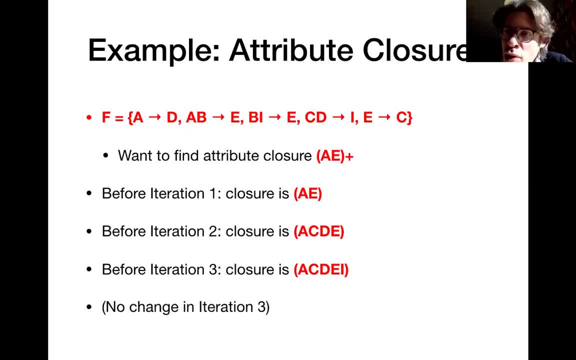 and that might mean that now more function dependencies become applicable. So if we go through the functional dependencies again this time, considering that we are given attribute values for attributes A, C, D and E, we can see that here we have the function dependency C. D implies I. 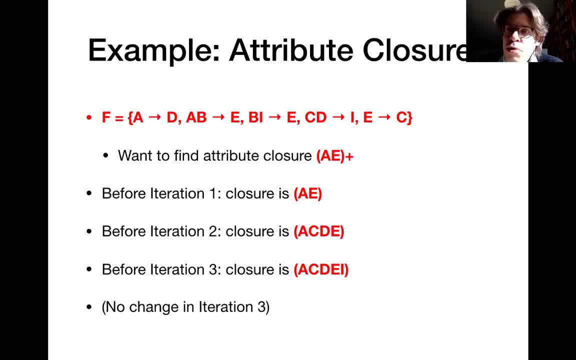 So if you know a value for attribute C and the value for attribute D, then you can infer the value in attribute I for the corresponding row. So because of that, we are adding I into the closure as well. All right, And so. 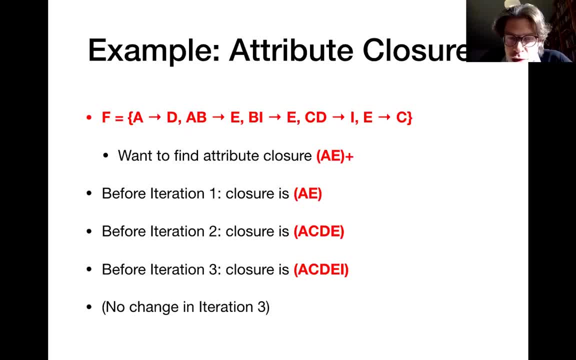 here we have expanded the attribute closure to A, C, D, E, I. Now, when going again through the function dependencies here, A B implies E, but unfortunately we don't know B. B I implies E, but we have already E and we don't have B anyway. 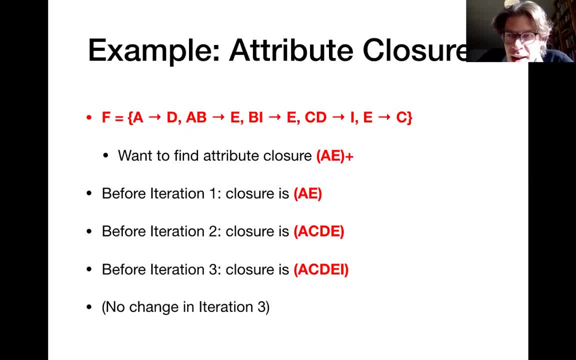 C. D implies I- All right, We have that. And E implies C- We have that as well. So here nothing really changes anymore by the next iteration, And this is how we know that we have converged. And now further iterations would not expand the attribute closure any further. 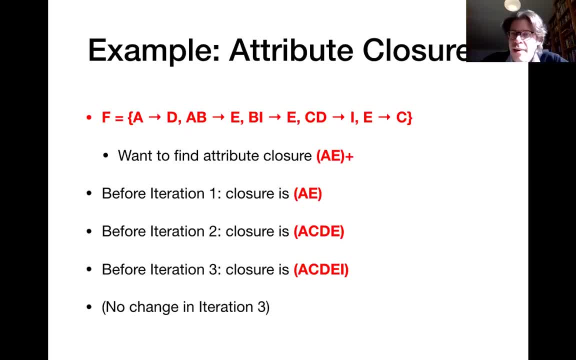 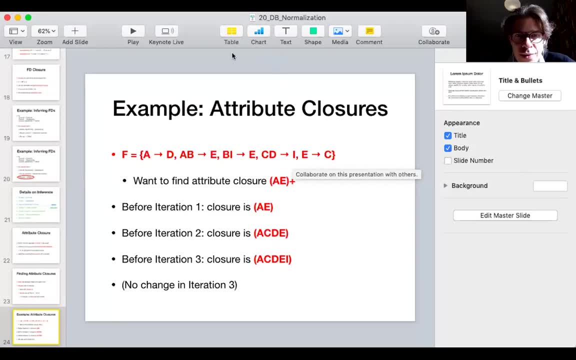 This is why we can stop the algorithm. Now we have calculated the attribute closure. I believe there might have been a question. Next example: Exactly Excellent, very good. So the question is whether this means that in knowing values for the attributes A and E. 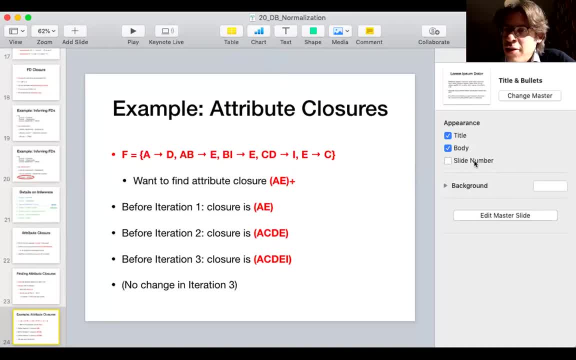 we can infer values for attributes A, C, D, E and I of the functional dependency. That is correct. So the attribute closure essentially gives you additional functional dependencies that can be inferred from the original functional dependencies. yes, So based on what we see here in the attribute closure, 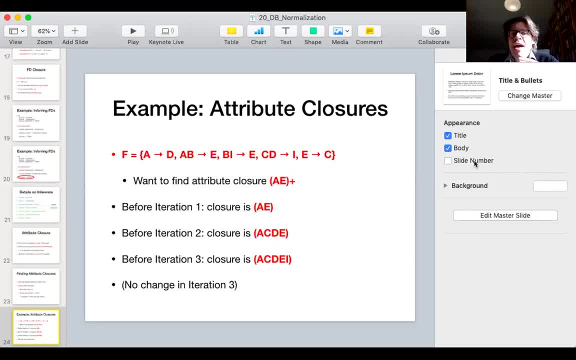 we know that we have the function dependency. A and E implies A, C, D, E and I or any subset of that. So the attribute closure generally gives you a subset of the total closure with a specific attributes on the left-hand side. 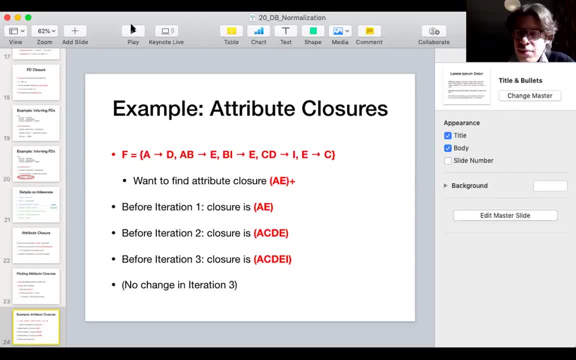 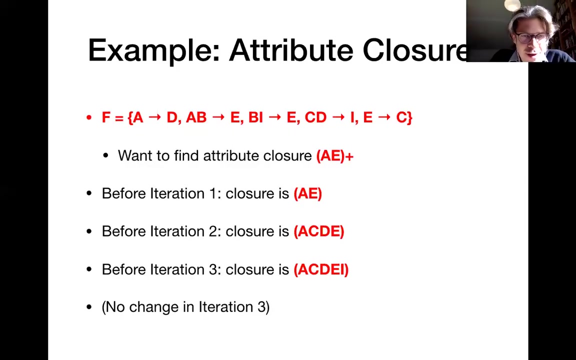 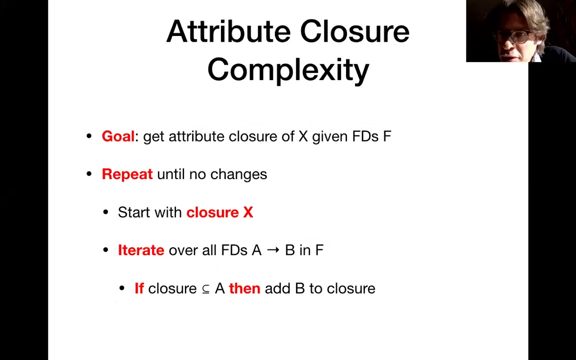 So yes, you are correct. Is there any more questions about the attribute closure at this point? All right, then Let's continue. All right, before we go further. first of all, I want to show you that this is actually a pretty efficient algorithm. 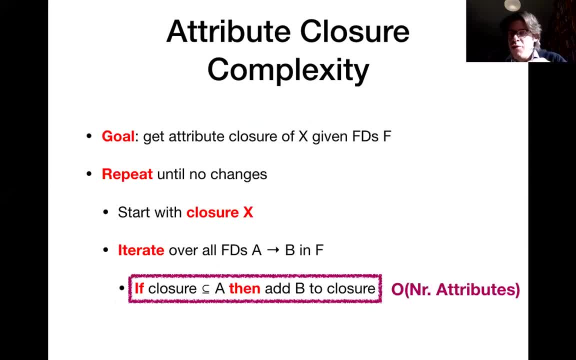 So here we have the algorithm again, And now we analyze the complexity Here, for instance the innermost command nested in those loops. here that one should have a complexity, OK, OK, OK, OK, OK, OK, Yes. 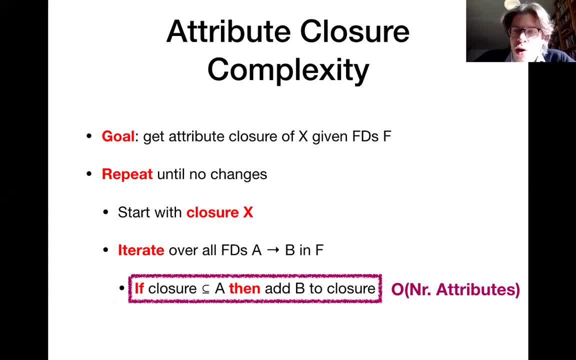 I understand. I guess that's fine. OK, so there's all of my questions now And I'll just in turn provide the last task, sharing some finaliff structure on this problem for slide two. OK, so this is pretty quick to do. 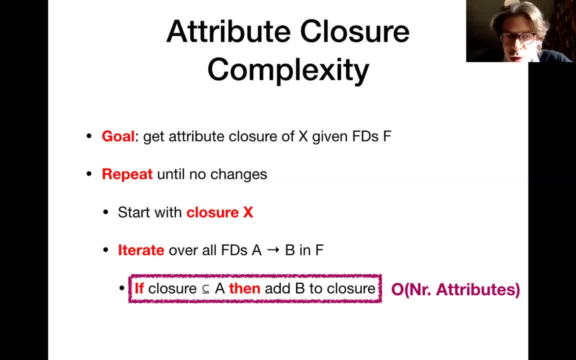 because you're correct, proportional, at most, to the number of attributes. So this is relatively cheap. but let's see how often we execute that. Here we iterate over all function dependencies. so clearly the complexity is proportional to the number of function dependencies And here, finally, we have a loop that keeps iterating. 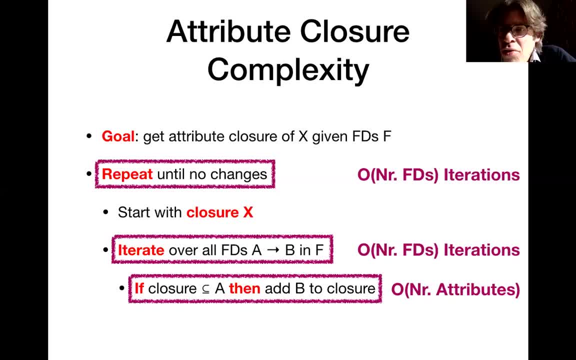 until a convergence. But we know that for each function dependency in my function dependency set it will only change the closure once, because if it has been triggered, meaning if the left-hand side of the function dependency is known, then we add the right-hand side of the function. 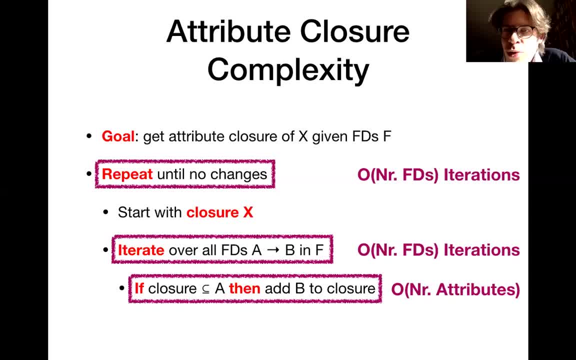 dependency into our closure, But it can only happen once for each functional dependency, and if you don't have any changes to the closure anymore, then we terminate our iterations. So because of that, I know that the number of iterations is limited by the number of functional dependencies as well, And taking everything together, I know that 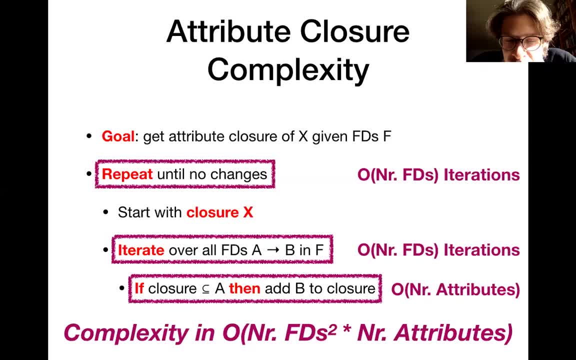 this algorithm is proportional to the number of attributes and quadratic in the number of functional dependencies at most, And this is already reasonably cheap, and so we don't have to worry about getting to the right degrees of just that. you know, there's also other algorithms that are even a little bit more efficient than 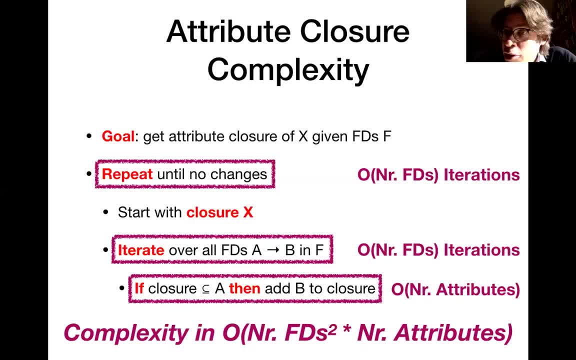 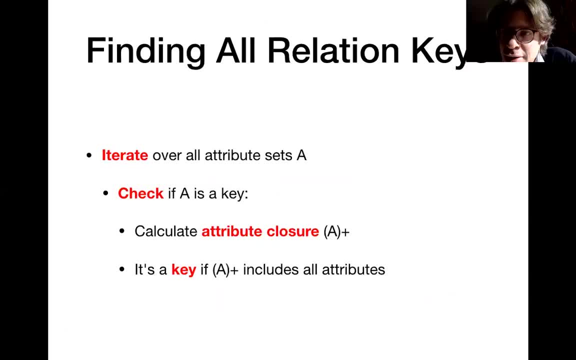 that, so the attribute closure can be calculated quite efficiently. one way in which we can exploit the attribute closure is for calculating all keys of a relation, and when discussing about redundancy, we have discussed that function dependencies- they can be good or bad depending on whether they have a key on the left hand side. so finding keys. 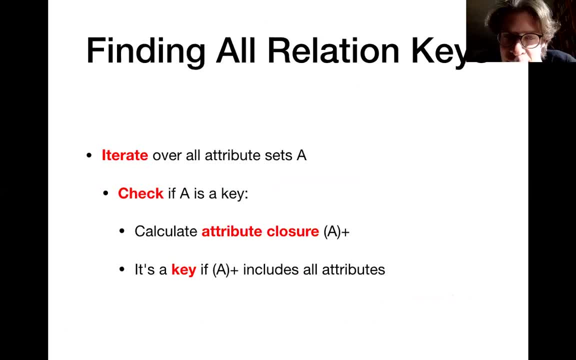 is generally important in order to assess a redundancy. and this is an algorithm that essentially finds all keys for a given relation. so if we simply iterate over all attributes sets of that relation, we can check if it is a key by calculating the x and we can check if the attribute closure for that attribute set and we have a key if the attribute. 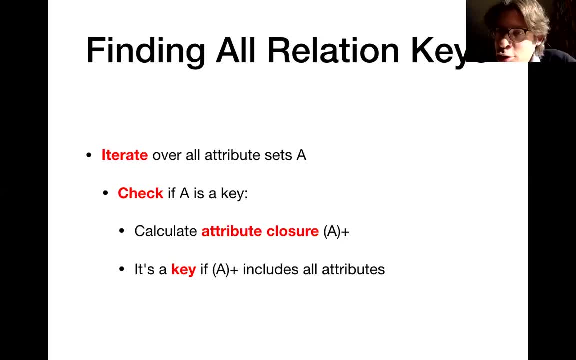 closure includes all attributes in the entire relation, because a key is essentially a special case of function dependency where the left hand side implies all the attributes in the entire table and this is what we can check using the attribute closure. so this is one possibility to calculate all the attributes in the entire relation. so, if you see, the algorithm is, of course, a more expensive. 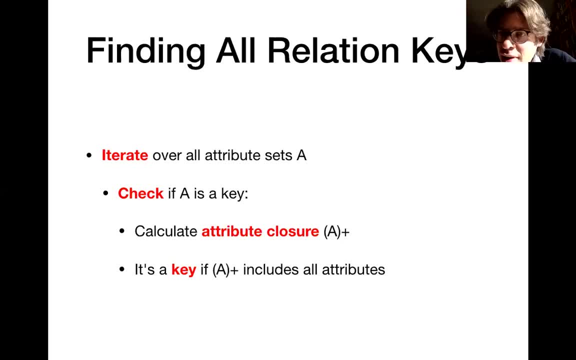 even though calculating the attribute closure is quite cheap here. this one iterates over all attribute sets, and their number is in general exponential in the number of attributes per table, so that is, on the other side, quite an expensive algorithm. all right, so, and just the same, typically, if you are calculating the attribute closure of a given relation, 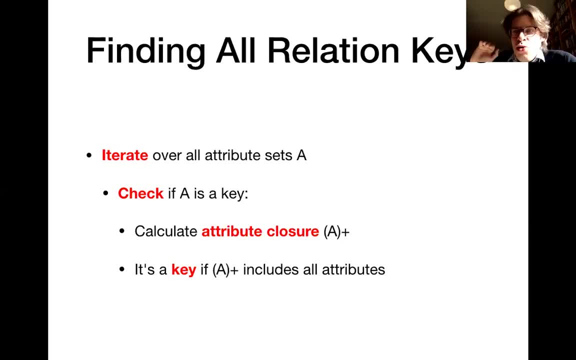 you are trying to get to a normal form, which we will do in a couple of slides. you don't have to calculate all the keys in the relation via this method. typically there's ways in which you can more easily recognize which function dependencies are okay or not. but in principle you could apply. 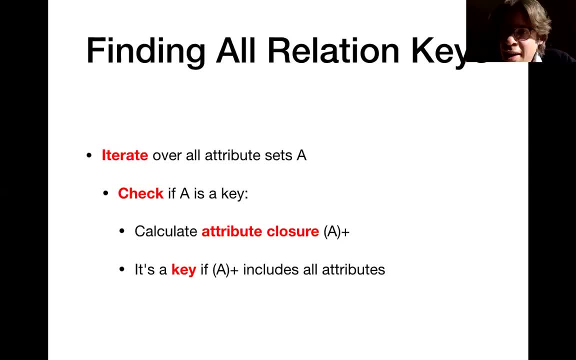 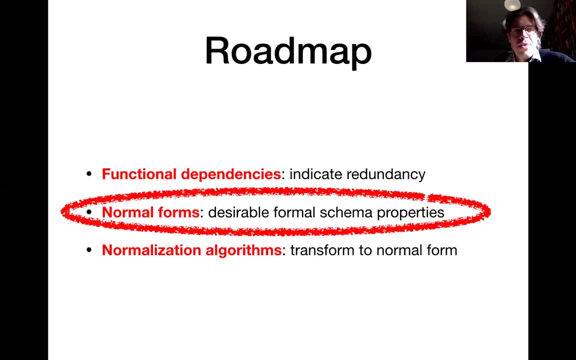 this one in order to get the full set of all possible keys, and that allows you to check whether function dependencies are okay or not. okay, all right. so now we have discussed the functional dependencies, we have discussed a couple of corresponding algorithms which allow you to infer functional dependencies, and next up is our 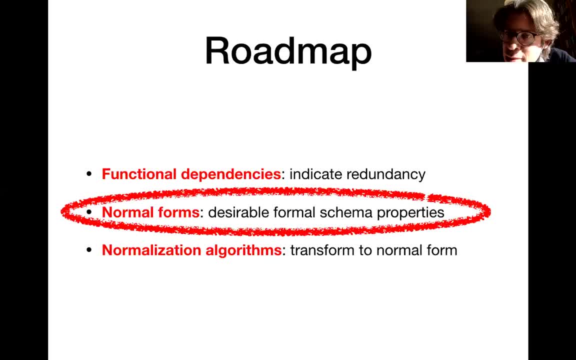 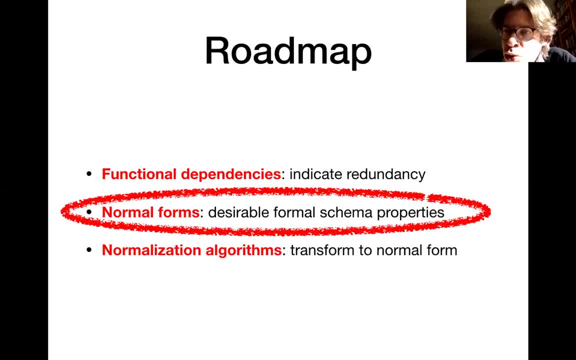 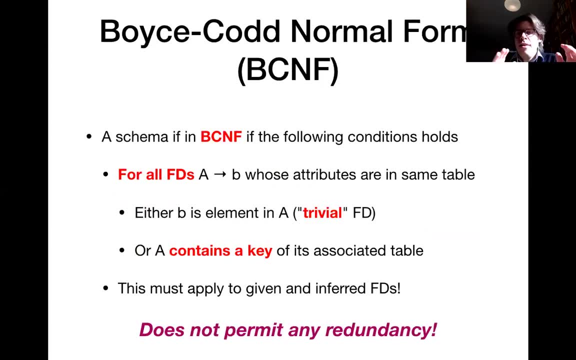 more normal forms from that are also used in practice. so here we are only going to cover the most important ones. one of those is the boy scott and normal form, short b, c and f, and in order to verify whether a given schema is in boyscott normal phone, you have to do the following. so here: 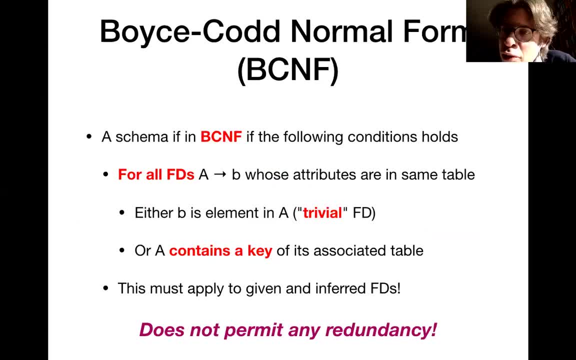 in the following: i assume that you have an overview of which function dependencies is called for that schema, either because of the main knowledge or because they can be inferred from initial functional dependencies, and also assume that you can assess whether a function dependency refers to a key or not. all right, so we decide whether a schema is in voice cut normal. 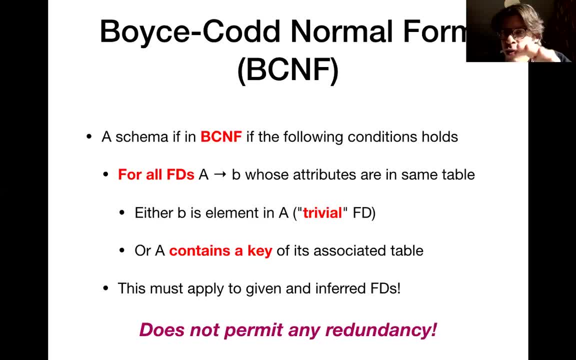 form by going for each table, over all the function dependencies which holds within that a table and for each of those functional dependencies, uh, one of two cases must apply. in those cases is what you have here: a function dependency does not indicate a redundancy. if, first of all, 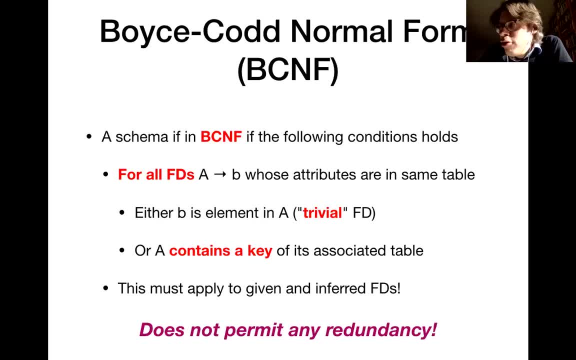 it is a trivial function dependency, and a trivial function dependency is something like saying that, um, knowing a value, knowing the name of the customer and knowing the age of the customer implies the name of the customer. we're just saying that knowing the name of the customer implies knowing the name of the customer. so those are trivial functional dependencies. they 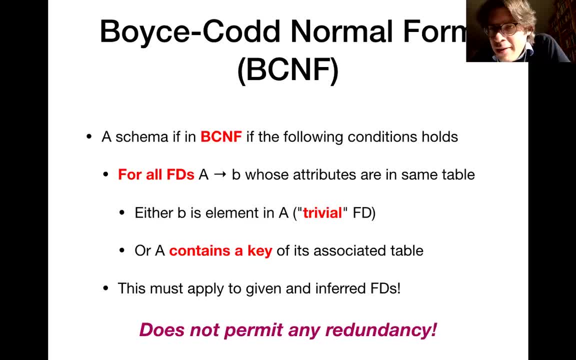 always hold and they don't specifically mean that there's any redundancy, so that is definitely okay. um, on the other side, function dependencies are okay if they represent a key constraint, meaning that the left hand side implies all the attributes in the entire table. key constraints are okay because for the same values in the key columns i cannot store any. uh. 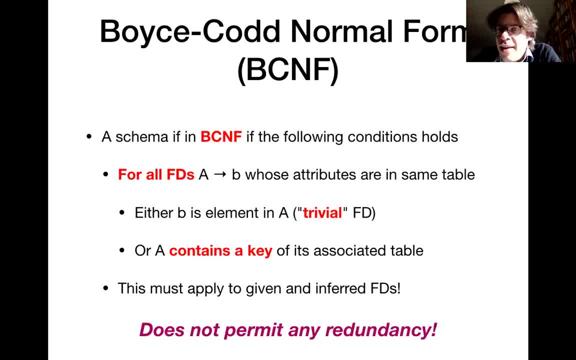 two, any two rows. so because of that i know that there won't be any redundancy. and if for each functional dependency on a table both of one of those two constraints applies, um, and if that holds for all the tables in the database, then the corresponding schema is said. 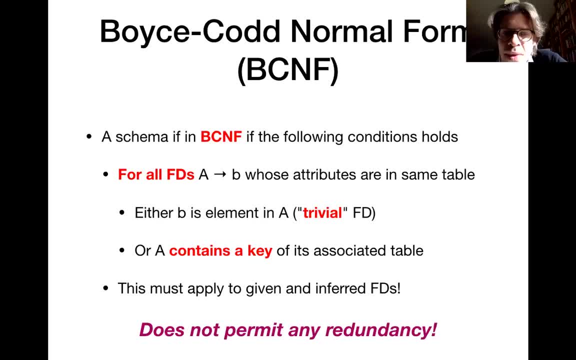 to be in boy scott normal form. so this is very strict about avoiding any redundancy. okay, and here there is a question. i see whether a, b is a set or a single value. okay, great point. so in this case, um, we assume that we have normalized the function dependencies. 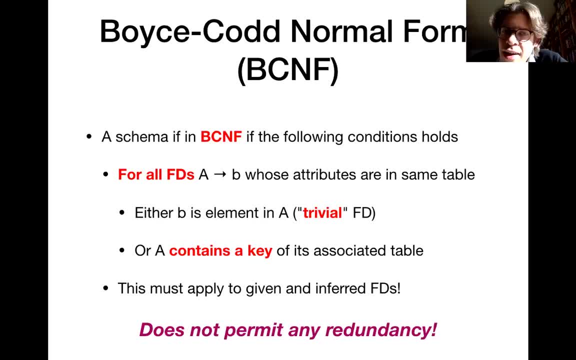 and put a single value on the right hand side, you can show that you, if you guarantee this for those function dependencies, then it will hold in general. okay, so very good point as picking up on that. yes, so here we essentially assume that we have a single attribute on the right hand side. 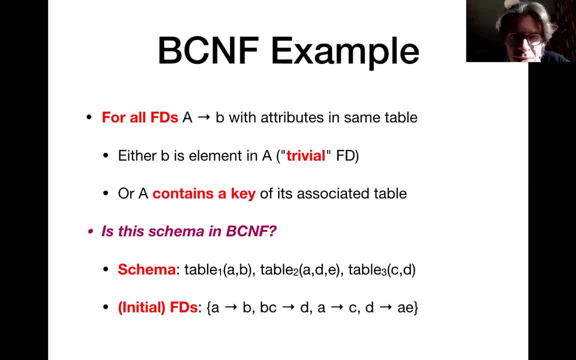 let's make a little example to make things more concrete. we have a schema given on the lower side of the slide and i have given you the shorter version of the definition of the boy scott, normal form, on the upper half of the slide. here we have 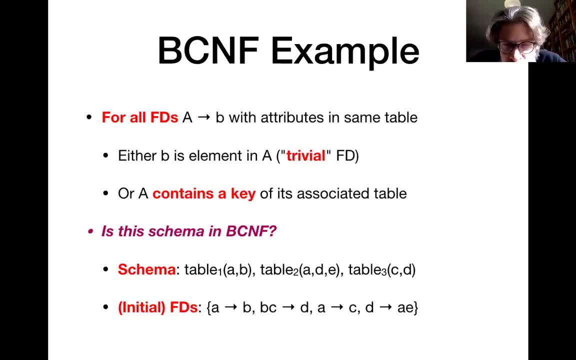 three tables in the schema which have different subsets of attributes and we are given the function dependencies that you see here on the bottom of the slide. um, does anyone want to tell me whether, um, whether, we might have a boy scott normal form here? so fancy what we get from the default tables in general. 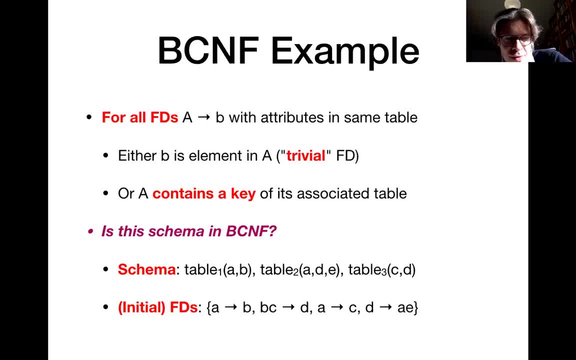 however, number one, which has the attributes A and B. Does anyone want to make a guess about whether this table satisfies the conditions for Boyce-Codd normal form? Yes, very good. So A implies B is okay, because A is the key for this table. 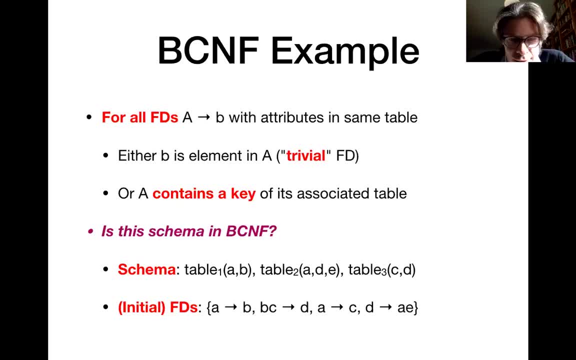 So we have one of the two cases that we want. Very good, okay, Let's maybe treat the third table before the second table, because the third table has less attributes. It has only attributes C and D. I believe there's a follow-up question in the chat. 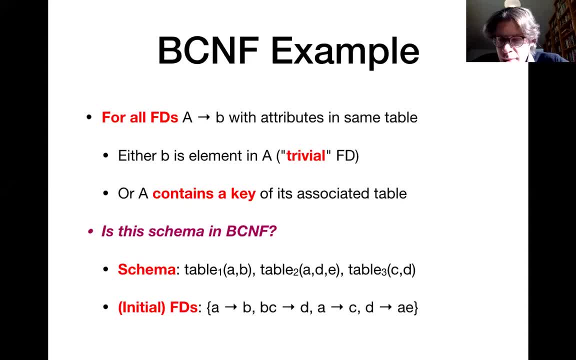 How do we know if something is a key in this example? Well, the definition of a key is that, essentially, by knowing the value of the table, by knowing the values for those columns, you can infer the values for all columns in the same table. 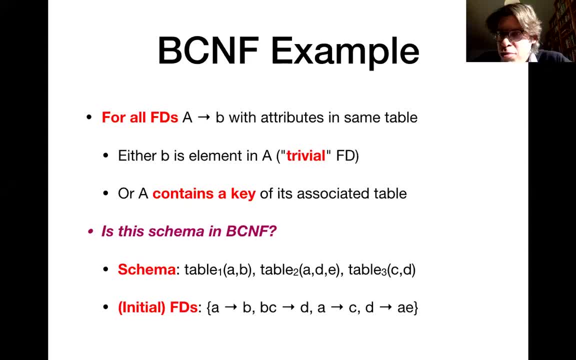 And in this case, for table one, you only have two attributes, which is A and B, and we are given a function dependency which says A implies B And because of that, I mean this is a function dependency that holds on the attributes of table one. 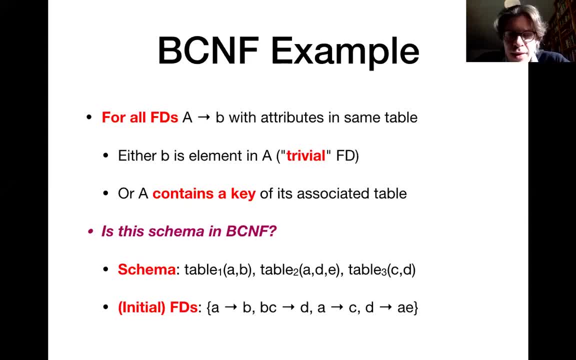 So we have to decide whether it represents any redundancy or not. but since here A is a key, a key, it means that this functional dependency is okay. so this is implied by the function dependency. a implies B and a key that always relates to one single table. so in order to be a key, it 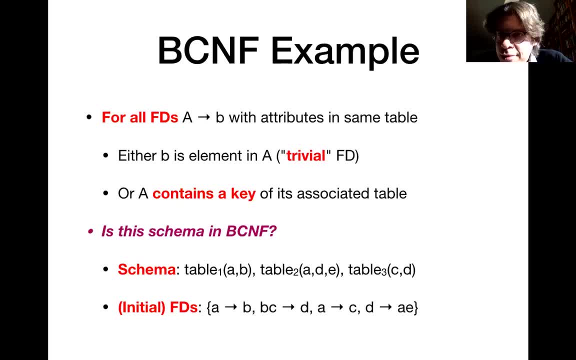 only has to imply the attributes that are in the same table. great question, all right. anyone has any suggestions about table three? table three is actually also, it's quite. table three is actually also, it's quite. table three is actually also, it's quite non-negative, dangerous in a way, because here we only have a two attributes. so if there's a functional dependency, 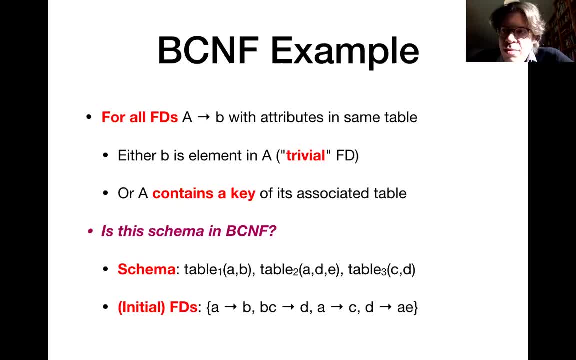 that is a non-trivial, then it essentially must be of the type that knowing the value in one of those attributes implies the value in the other attribute, because- but because we only have two attributes, it means that in that case it would have to be a key as well. 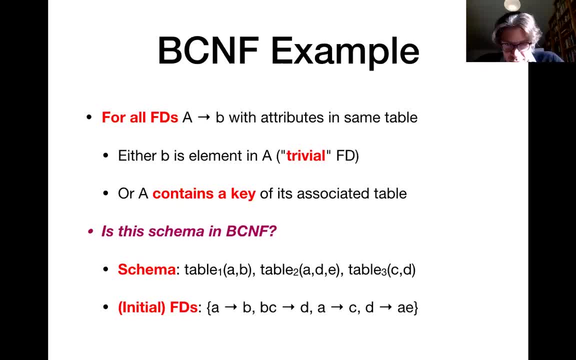 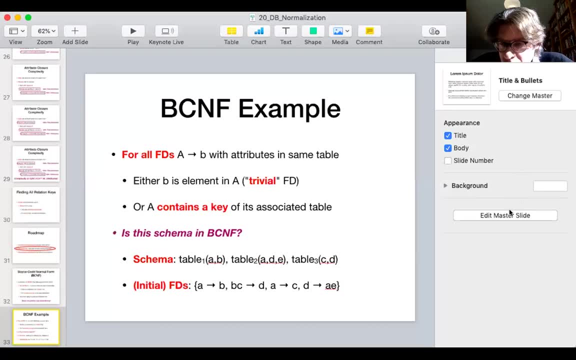 so here, um, there is a, no specific uh functional dependencies and quickly, quickly moving this, so there's no specific function dependencies with c here. on the other side, d implies a and e, and and a implies a c. so d implicitly implies a c as well, but um here that makes it a key. 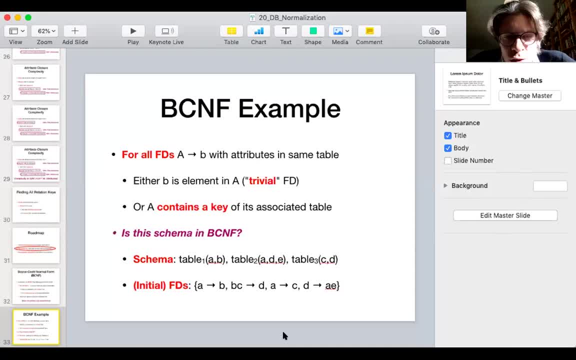 and therefore we don't, we don't violate the constraints of boy scott: normal form. and here, that was exactly the comment i see here. yes, exactly yes, you're absolutely correct. that was exactly the comment i see here. yes, exactly yes, you're absolutely correct. eat, that was exactly the comment i see here. yes, exactly yes, you're absolutely correct. d is a key here in table three. 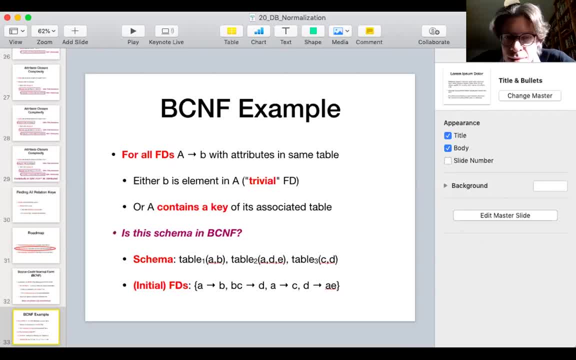 because, um, it implies c. very good, okay, so that table is also okay now. very good, okay, so that table is also okay. now let's finally look at table two. um, it has attributes ad and e. so anyone any suggestions about that? so anyone any suggestions about that? 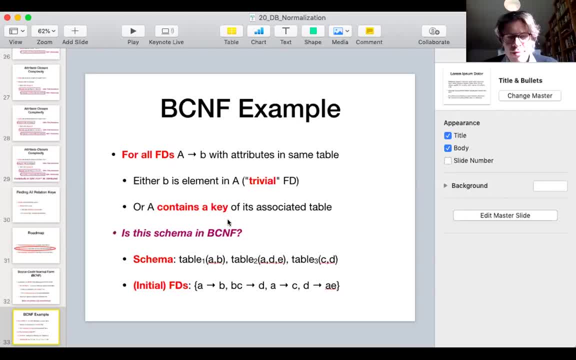 can anyone spot a key for this table? okay, d applies a and e. yes, very good, absolutely so. d is definitely a key. see any other keys. very good, yes, exactly so. over a couple of corners. a also implies all the other attributes. see here. a implies a, B and a. 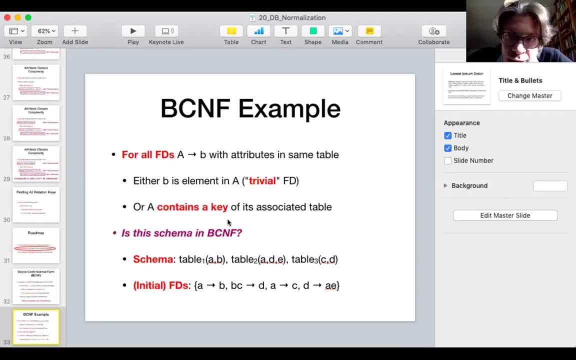 implies a C and BC implies D, so aim plies a key, which means that it also hotel bar as well. the right hand side a key via transitivity. yes, so a is also a key here, right, so also all function dependencies that have a on the left hand side should be fine or function. 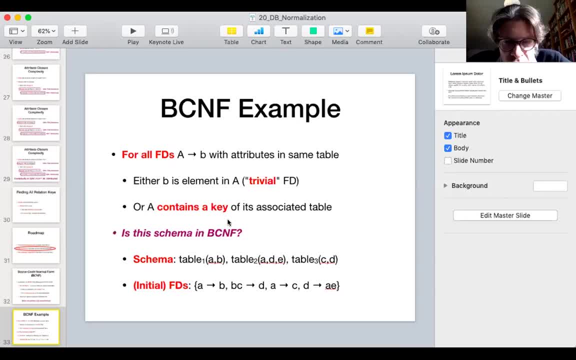 dependencies that have D on the left hand side should be fine, and here, finally, e, there's no real function dependencies which have e on the left hand side, so here it seems that all the function dependencies are okay and therefore this should be in a Boyce caught and normal form. all right. 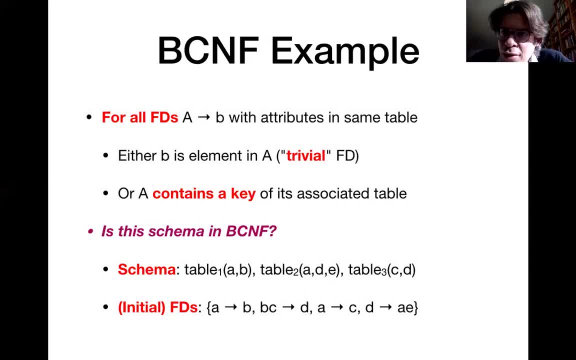 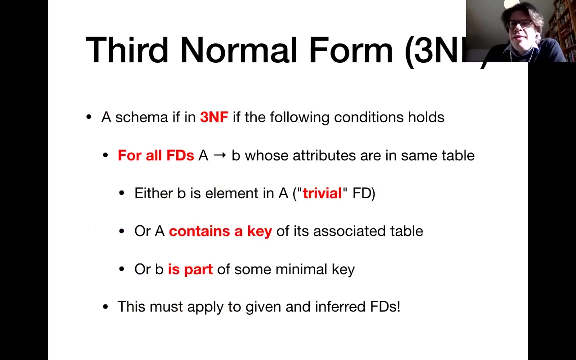 yes, exactly so essentially you're checking for all the function dependencies that can be inferred from. the original function dependencies question was whether a Boyce caught. normal form considers the entire closure of function dependencies and yes, that is the case. all right now the second or the third normal form here, but the second one that 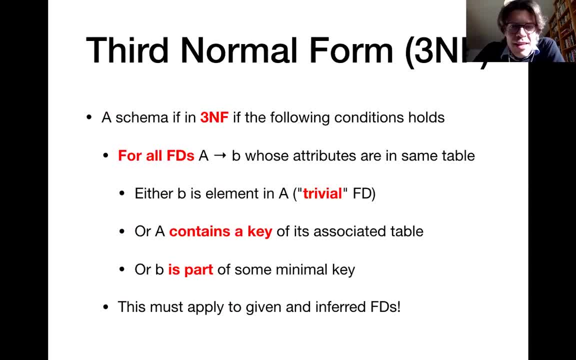 I'm discussing in this lecture here. that is the one that you see here and that is another very commonly used normal form. in practice it is a little bit more perma- missive compared to Boyce caught normal form, because here for each of the function dependencies we require not one. 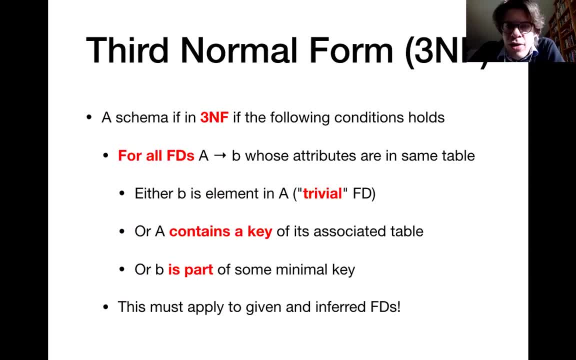 out of two, but only one out of three conditions to be satisfied, and the first two conditions are exactly the ones that we have seen for the Boyce caught normal form. so when going over all the function dependencies that hold for a specific table, we say that they're okay if they're either trivial or 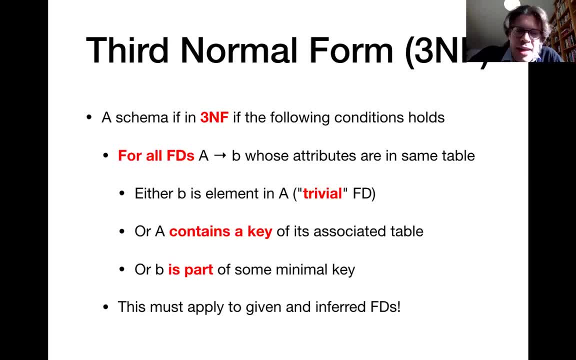 or if the left hand side contains a key or if the right hand side is part of some minimum key for the relation, and the minimal key is generally it's a set of columns which forms a key, but if you take away any of those columns, then you won't have a key anymore. so this is essentially a key without. 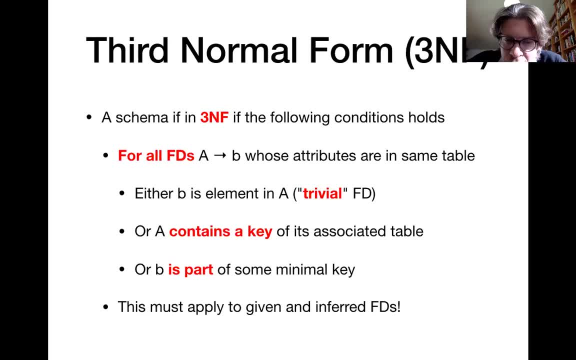 any redundant columns added to it. all right. so again, the process to determine whether a given schema is insert. normal form is to go over all tables, for each table to collect the function dependencies- initial or inferred doesn't matter- all the function dependencies which apply to the attributes of that table, and then to check for each of them whether at least one of those conditions 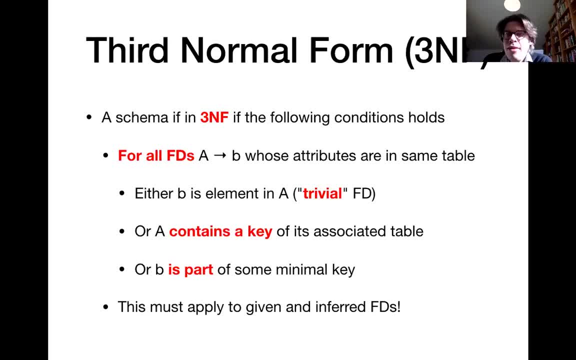 apply, and if that applies for all function dependencies and for all tables, only then is the corresponding schema in assert a normal form. all right, and a minimal key is generally a key, which stops being a key if you take away any columns. so you have a set of columns. 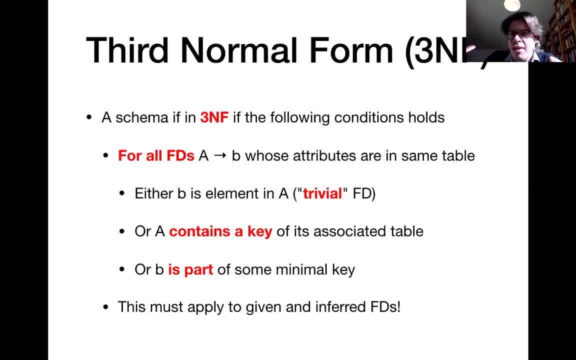 which imply values for all the other columns in the same table. but if you take away any of those columns then you cannot do that anymore. a key without any superfluous, without any redundant columns, all right. so this assert condition is new compared to voice code normal form and it allows a certain 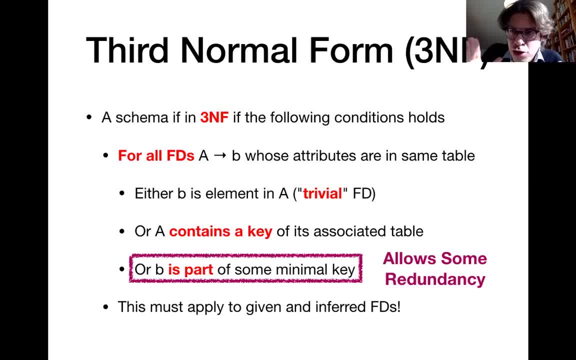 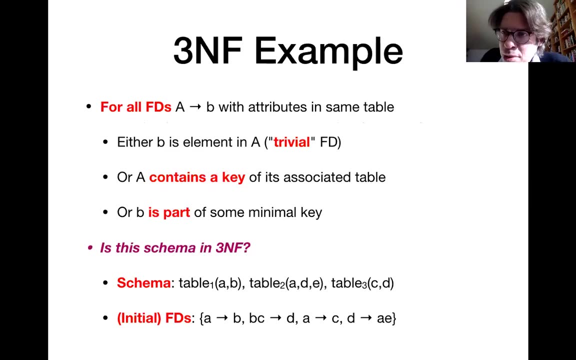 type of redundancy. so this is a very specific condition here, of course. so one might wonder why people allow specifically this type of redundancy. and um, before we go into this, i'm going to tell you a little bit more about that on the next slide, but let's already make a little example for verifying whether something 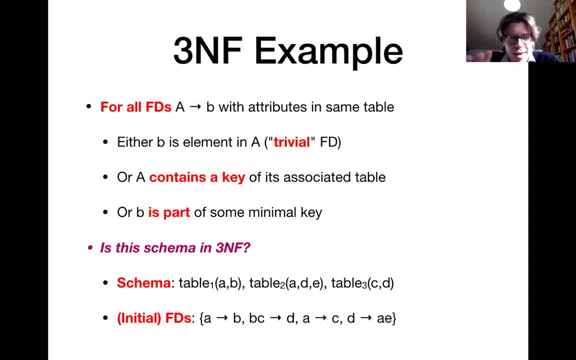 is in the subnormal form. and here we have the same example again. so can you tell me whether that is in subnormal form? yes, exactly, very good. so here the insight is that, uh, voice code normal form is essentially a restriction of start normal form. so if 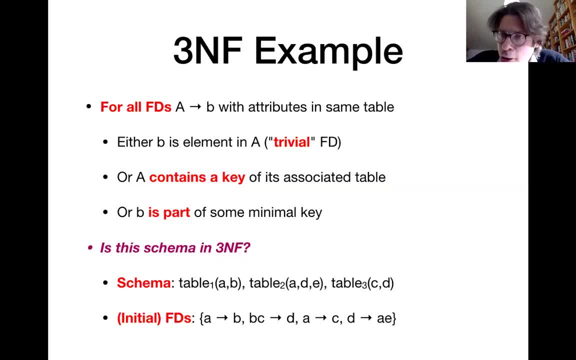 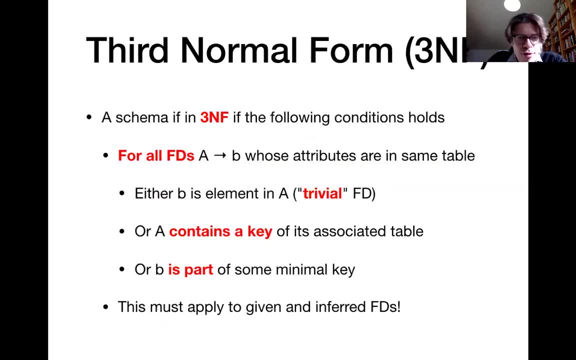 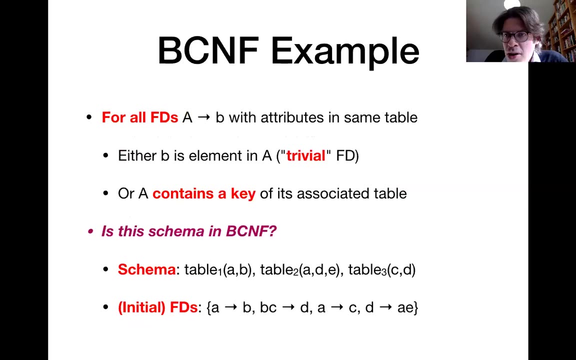 something is in boy scott normal form, it also must be in certain normal form, because if you compare the conditions, you can quickly do that again. if you compare the three conditions of third normal form and the two conditions of boy scott normal form, the first two are essentially identical. so 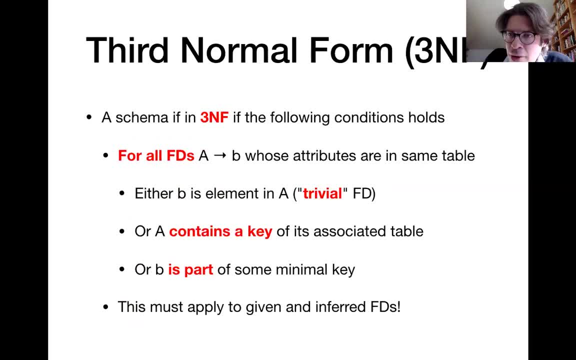 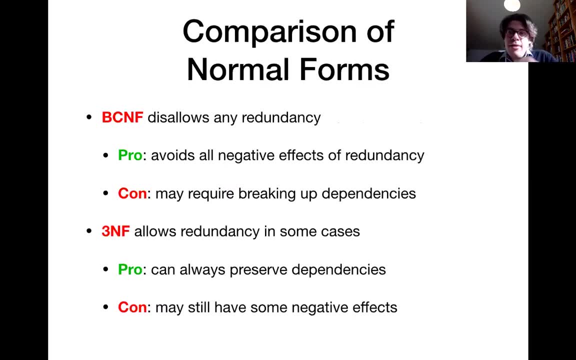 third, normal form is really just a little bit more permissive compared to boy scott normal form. all right, so if we compare those in normal forms then i mean at first one could think that boy scott normal form must be better because it allows less redundancy. we have seen that redundancy. 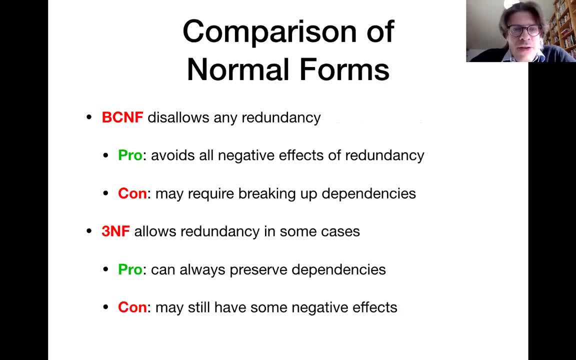 has quite a few disadvantages. so, um, that is the advantage of voice code normal form, that we don't have a redundancy anymore. on the other side, um, it also has a disadvantage, because we have to break up our dependencies, and that means, essentially, the first one is a good. 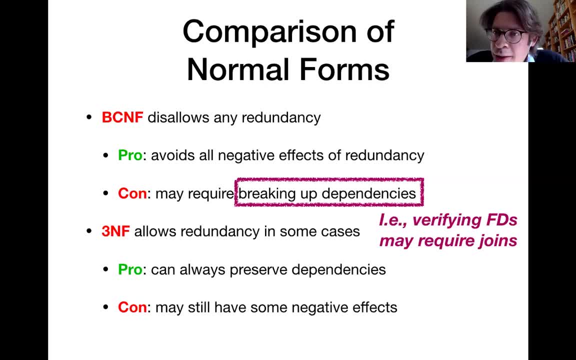 the following: If you have functional dependencies, then you often want to verify that freshly inserted data satisfies those functional dependencies. For instance, in our original example we had a function dependency linking the number of hours worked by TAs to their salary. and if I would now try to insert 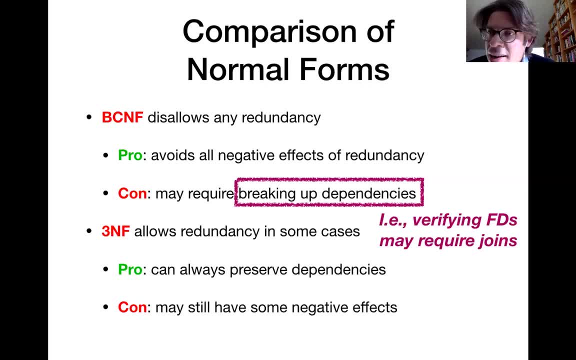 a new TA into the database with a salary that is inconsistent with the number of hours worked, then I probably want to reject that update and in order to verify whether that update is okay or not, in some cases I might actually have to look at multiple tables and I might have to join them in order to verify. 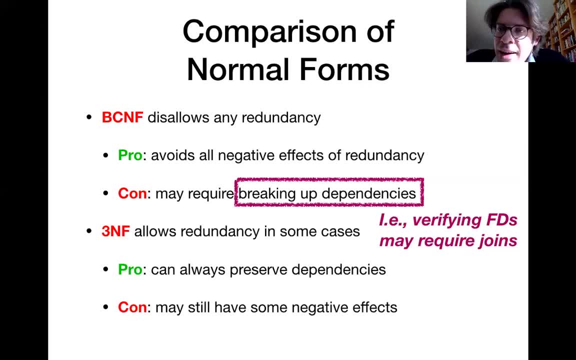 whether a certain functional dependency is satisfied, And the drawback of Boyce-Codd-Normal form is essentially that I might have to decompose tables so far that in order to verify some relevant functional dependencies, whether they hold for new data, I might have to actually join. 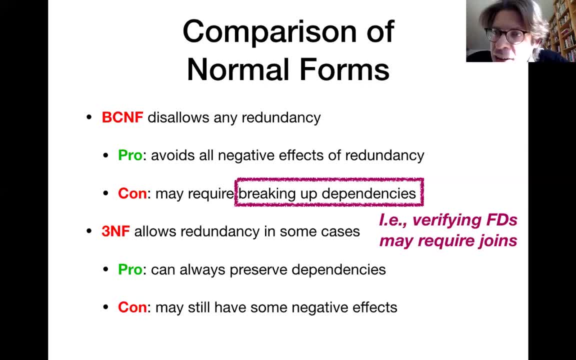 multiple tables together and, as we know, the joins are expensive and therefore you might want to allow a little bit of time to decompose tables, To allow a little bit of redundancy, if it helps us to avoid additional joins. and this is exactly what the third normal form has been designed for, so to speak. 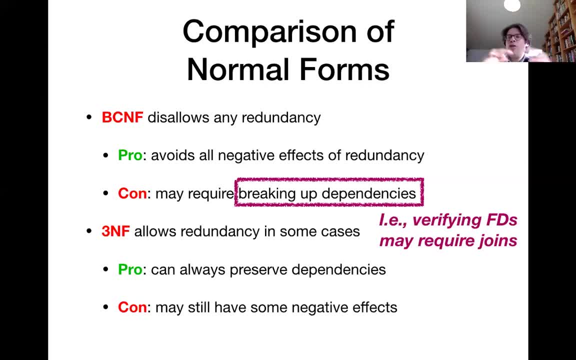 It allows us to always preserve dependencies, meaning that I can verify functional dependencies without having to do any joins, and this slight extension of Boyce-Codd-Normal form you can prove, even if we are not gonna do it here in the lecture. So I'm going to show you how to do it. 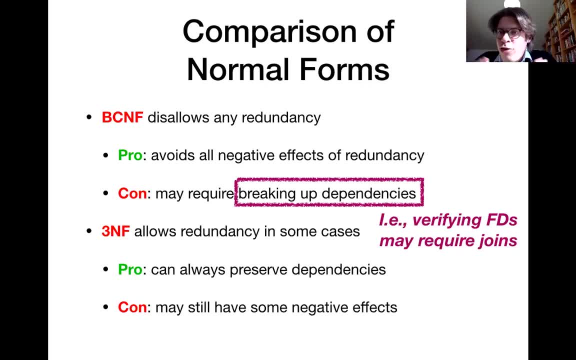 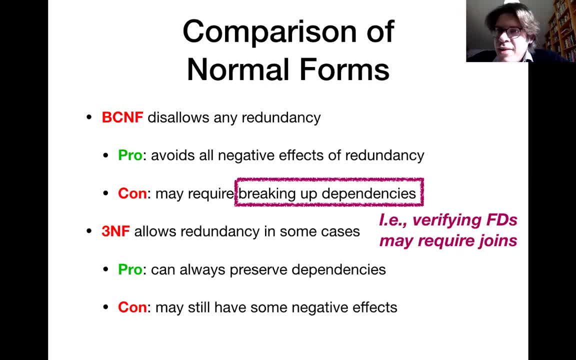 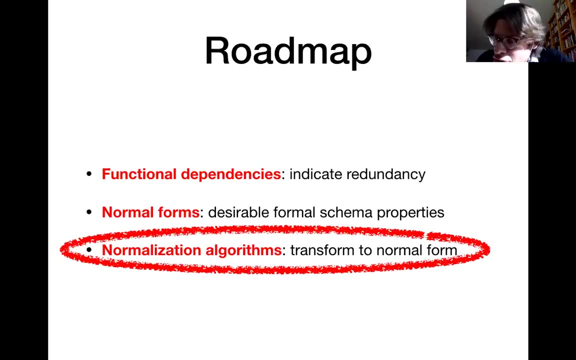 have a look into the book, into chapter 15.. But this is the reason why we want to slightly relax the requirements of Boyce-Codd-Normal form. Alright, so those were already the normal forms that I wanted to introduce here, because those are. These are the only ones that I think are going to be used in this lecture. 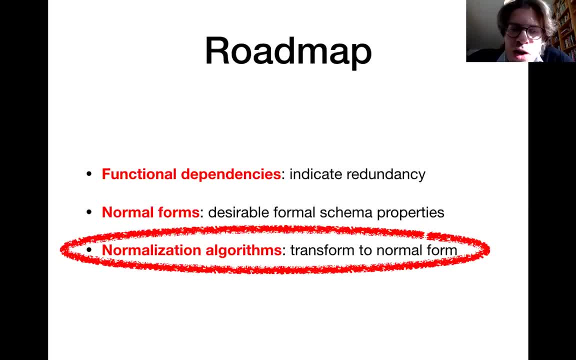 are two of the perhaps most popular normal forms are used in practice. Now we're gonna start discussing a little bit about transformation methods And towards the end I can also take a few questions on some of the prior material, So the algorithms that we discuss here. 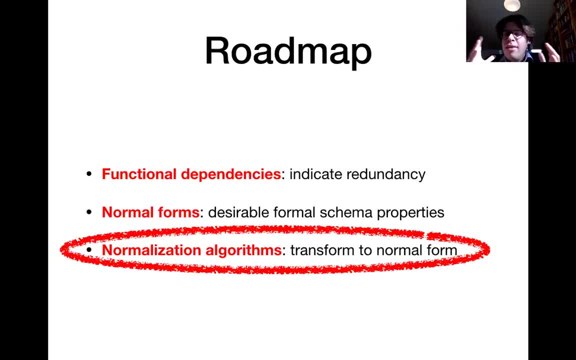 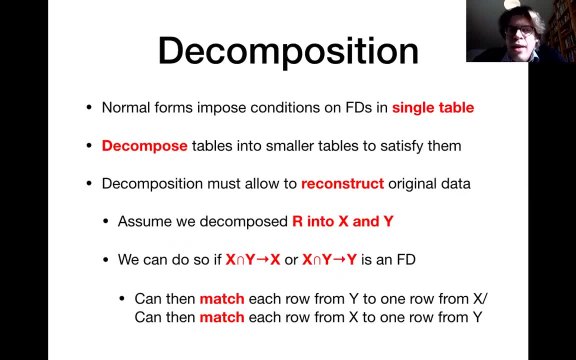 their goal is essentially to bring some initial database schema into one of those normal forms. And the way to get to some of those normal forms that is generally decomposition, and which is what we have already applied in our very first example, where we first had the TA name. 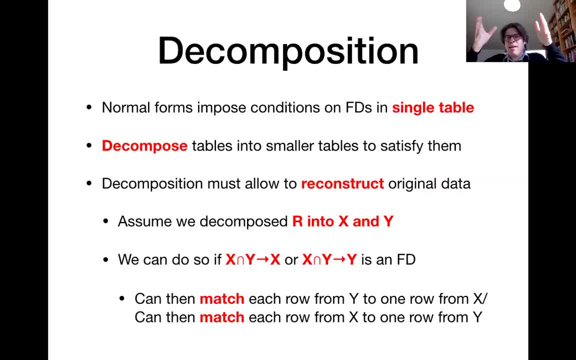 the number of hours worked and the salary in the same table, which caused problems. So we decomposed it into one table about TAs and the number of hours worked and a different table which keeps track of the relationship between the number of hours worked and the associated salary. 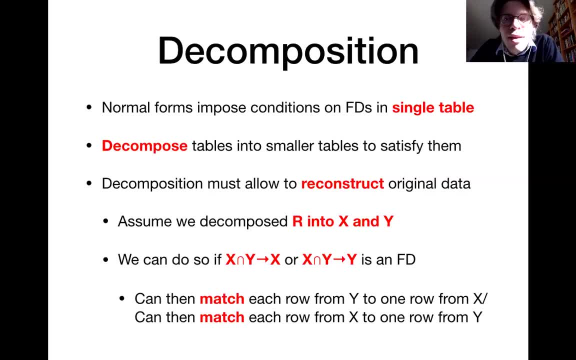 So the way to reduce redundancies is by decomposing those tables. One very important requirement here is that we want to decompose tables in a way that allows us to reconstruct the original data. We want to avoid redundancy, but of course we don't want to lose any data. 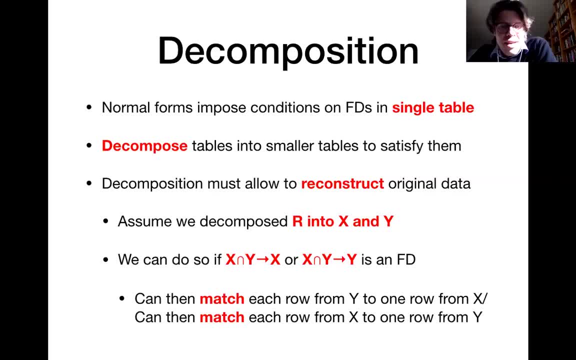 And the condition in order for this to hold is the one that you see here. So let's assume I have some relation R, where R is essentially just a set of attributes that relation has. Now I'm decomposing the set of attributes R. 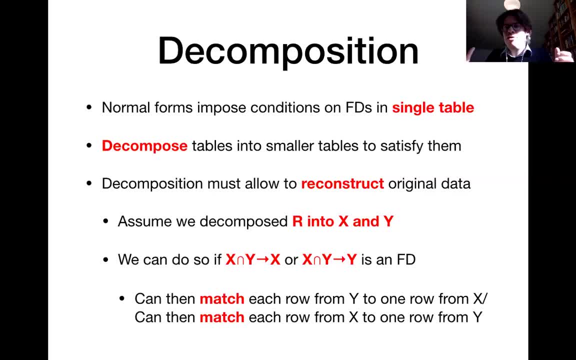 into X and Y and introduce essentially tables for storing those attributes in X and another table for storing the attributes in Y. Now X and Y they might overlap and if I take the union of them then I need to go back to R. 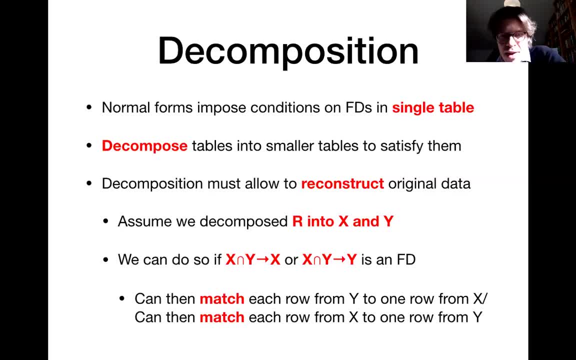 And I know that my details are perfect. now I need to change them And I need to go back to R. And I know that my details are perfect. now I need to change them And I need to go back to R. decomposition is okay if I know that intersecting x and y either implies all the attributes in x. 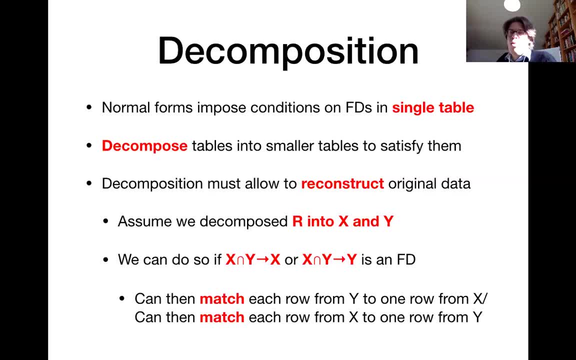 or all the attributes in y. Now what that means essentially is that if I join together the two tables after decomposition again, and I require that values are equal for those columns which appear in both of the decomposed tables, then if one of those conditions here holds, it means that 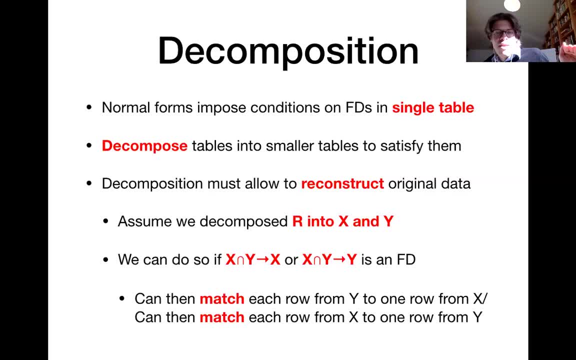 I can match each row in the table associated with x to exactly one row in the table associated with y or the other way round. So essentially, when intersecting those two column sets, then you need to obtain a key for one or the other of the two decomposed tables. In that case, if I do a natural join between the two decomposed tables, 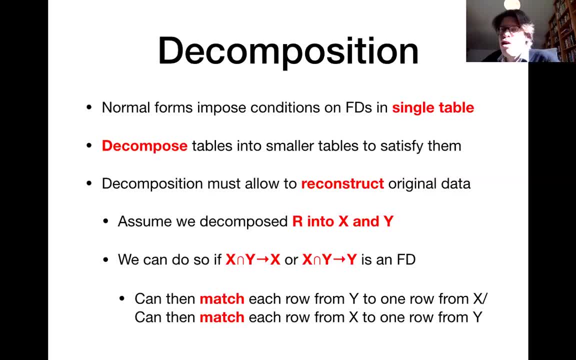 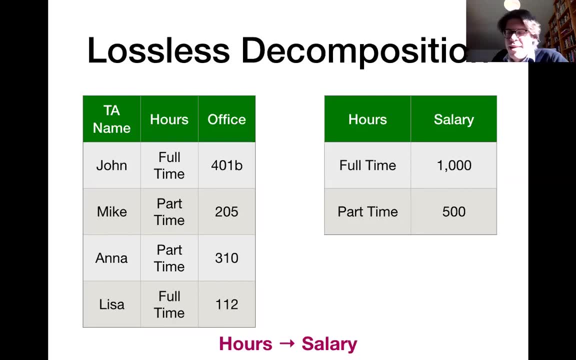 I will get back my original relation, which means that the decomposition is lossless. Now let's see a little example here. So here we have a slightly extended example from the one that we have originally seen. So here we have also added the office of the TAs, and again I have this constraint that hours implies the salary. So here, if I 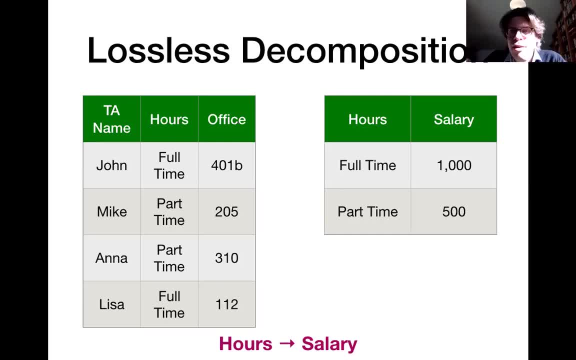 have decomposed my table into those two tables that you see here. you see that there is some overlap between the columns of those two decomposed tables. The hours column appears in both of them and if I do a natural join between the two decomposed tables I will get back my original relation. 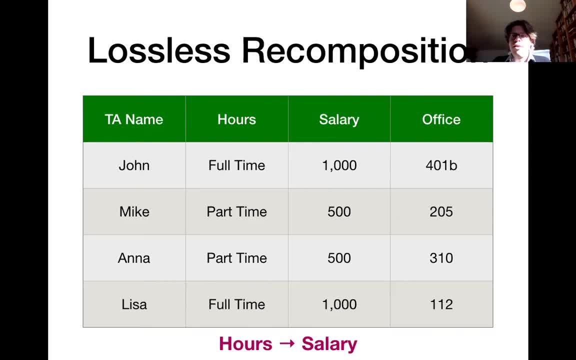 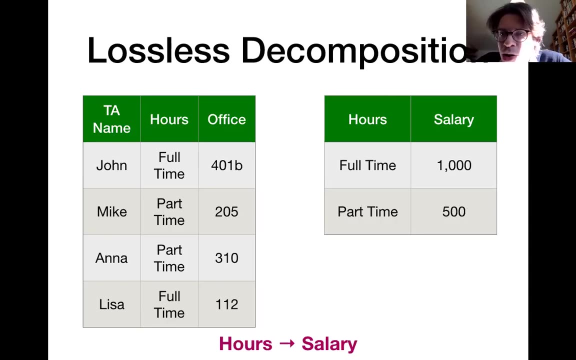 between them. What I will get back is this original table that you see over here, because the hours implies the salary and that means that for each row on the left hand side, I find exactly one matching row on the right hand side. So if I do a natural join between them, then I get back. 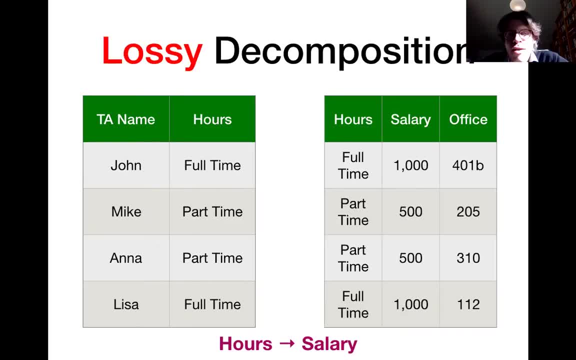 my original table. Now on the other side, if I decompose like this, I store the TA name and the number of hours in one table and in the other table I store the hours, the salary and the office of a corresponding TA. Now here that is a bad decomposition because I 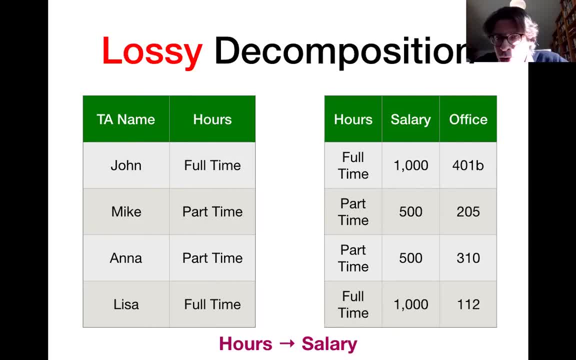 cannot really uniquely link rows from those two decomposed relations together again, because about the each TA, I will only know how many hours that a TA works. but the connection between the name of a TA and the office is unfortunately lost and if I would do a natural join between those two. 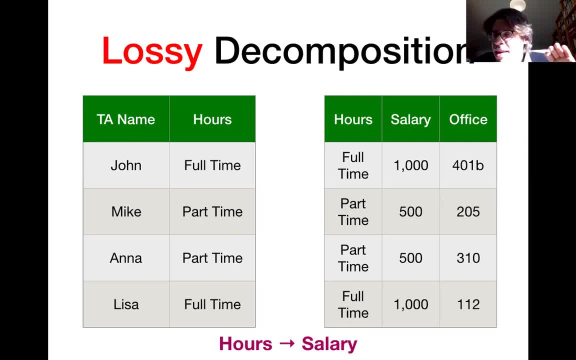 decomposed tables, then I would not get back the table that you have seen on the previous slide, but instead I would actually get back a larger table which has lots of spurious rows. I'm essentially combining one TA with the office of another TA which is working the same hours. 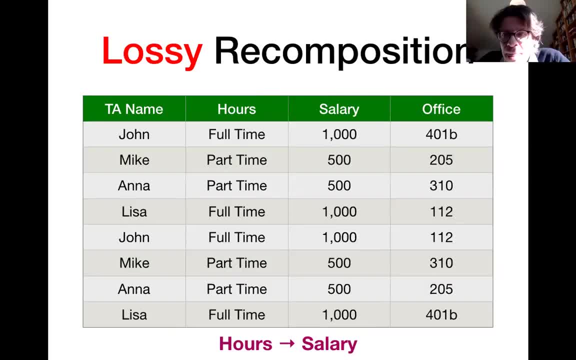 So here I would essentially get back this table over here. Now the name can sometimes be confusing. I'm calling it, or in general it is called, a lossy decomposition. but it actually means that if you would try to recompose things again, you would not get back less, but actually more than what you want. 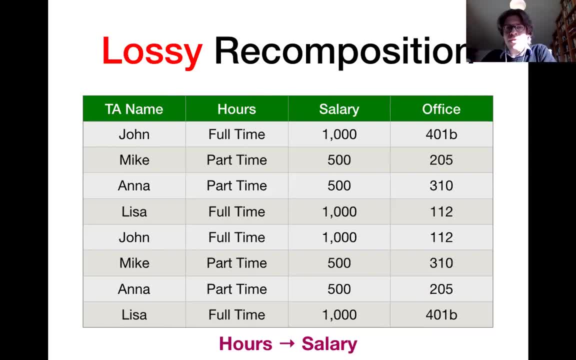 But that also means that information about which TA belongs to which office has been lost, and this is why we cannot get back our original data. So if I do a natural join between these two tables, then I would get back the data, which is bad. So this is how we want to decompose our TA. We want to make 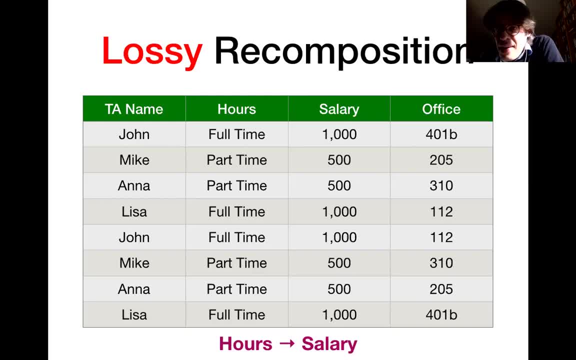 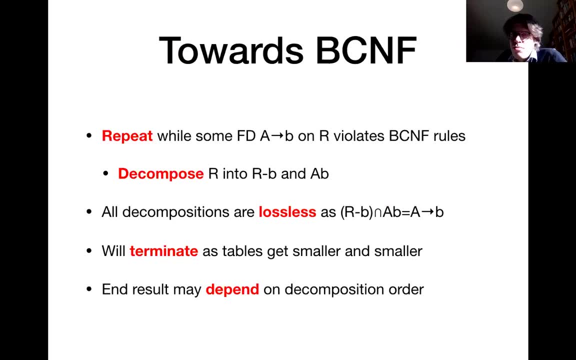 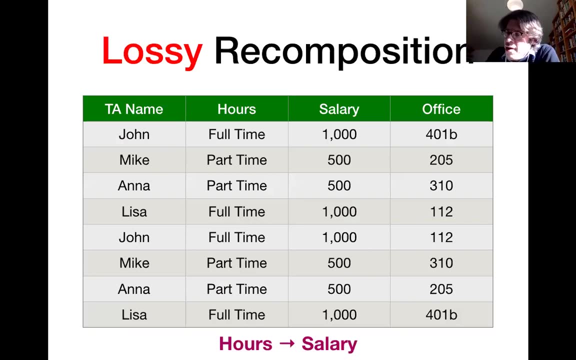 sure that we don't lose any data Now. the next time we're gonna see in more detail how we can use this decomposition method in order to get to one of those normal forms with a principled method. Now we have very few minutes left, so I can take a few more minutes. 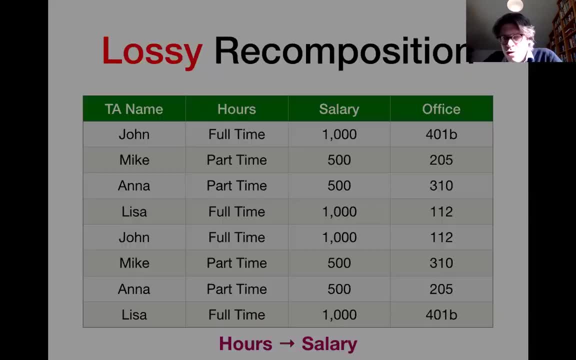 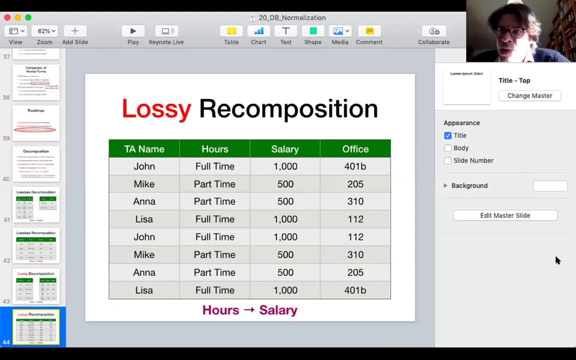 So let me take a few questions on some of the material. I think I had one at the very beginning. It was about when we release the locks of a transaction And how that relates to the commit time. So here the important point is that after you release the locks and before you commit, 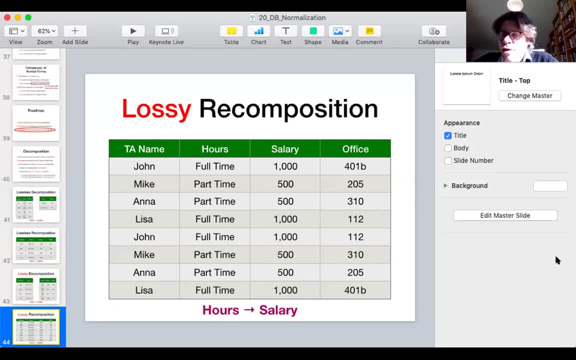 you can't allow any other transactions to grab locks on those objects on which you have just release the locks. if you want to be strict, because, um, the nice property of a strict two-phase locking is that we avoid those cascading aborts which can happen if a transaction releases the 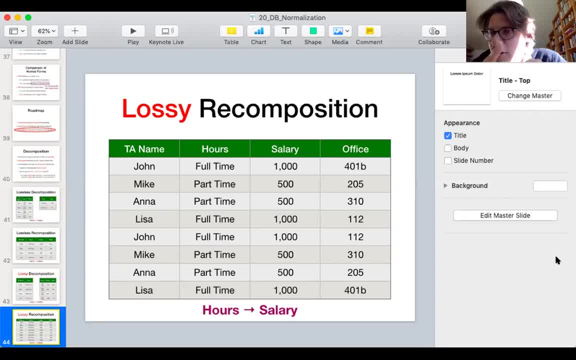 lock on an object early. then another transaction comes along and grabs a lock on that object and reads the current value. then the first transaction decides to abort. at that point it would also cause the second transaction to abort. so in order to avoid that, you want to make sure that between 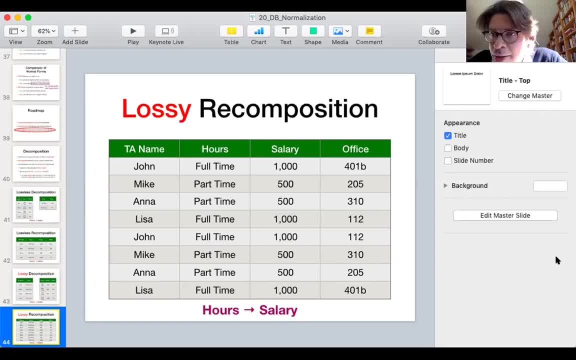 the transaction releases the lock and commits or a board. you cannot have any other transactions snatching the lock in between, so you want to get those two close together. yes, exactly. and for snapshot isolation: you abort if there is a conflicting rights on the same object. exactly, and for the.